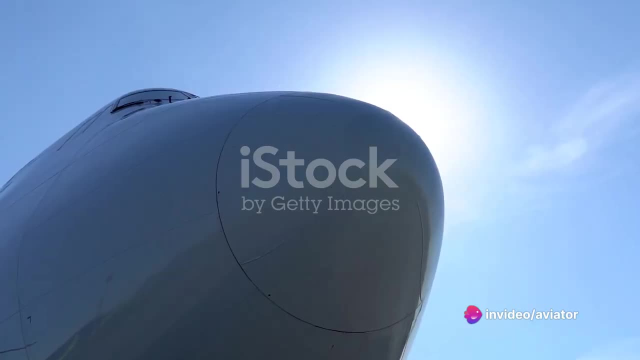 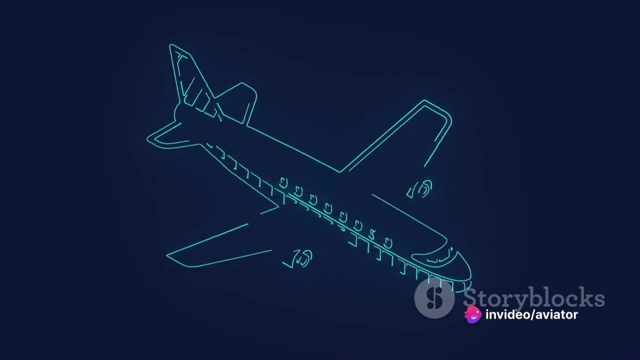 performance of flight, From the lightweight aluminum alloys that make up the fuselage to the robust titanium elements in the engine and the innovative composite materials that are constantly redefining the boundaries of aviation. These materials are chosen not just for their strength or weight, but for a multitude of factors, including cost availability. 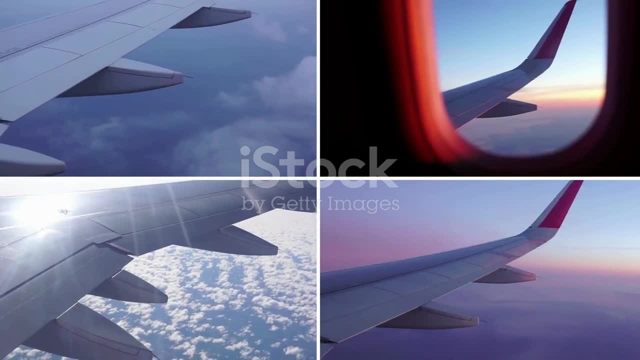 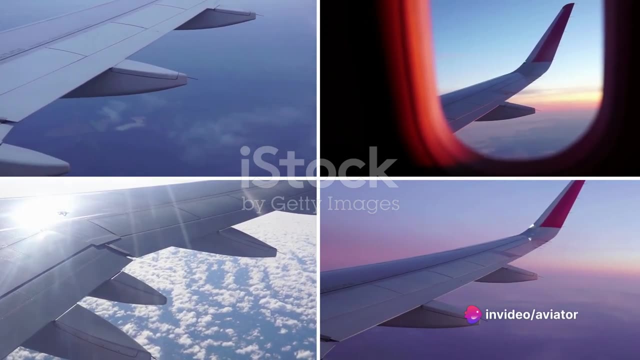 and their ability to withstand the harsh conditions of flight. So the next time you marvel at a jet slicing through the skies, remember it's not just the pilots or the engines that make it possible. Today, we'll uncover the secrets behind aircraft materials and how. 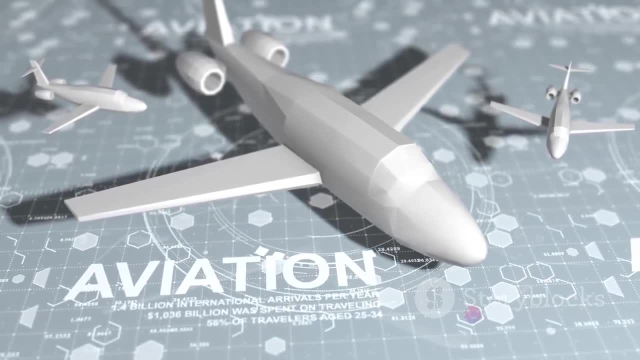 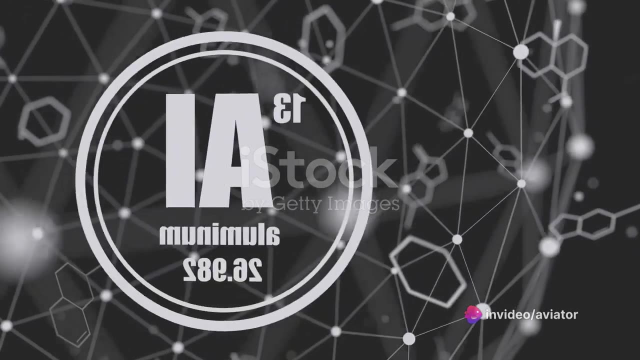 they influence everything from fuel efficiency to structural efficiency. In the past, up to 70% of an aircraft was made of aluminum. You might be wondering: why was aluminum so popular? Well, the answer lies in its unique properties: It's lightweight. 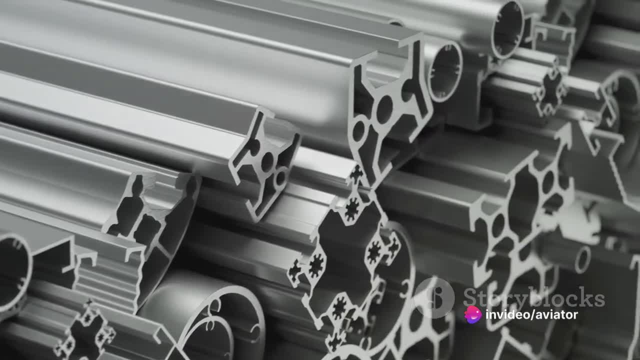 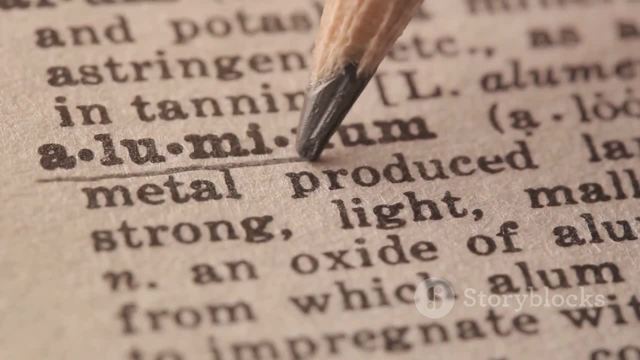 and inexpensive, which makes it a practical choice for large-scale manufacturing. Plus, it's widely available, meaning that manufacturers never have to worry about running out of it. Aluminum is like the reliable workhorse of the aviation industry. It's not the fastest. 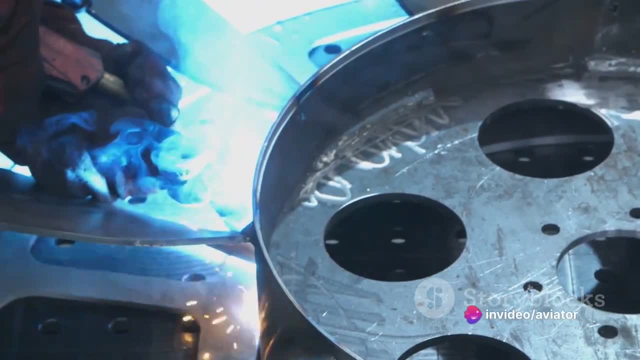 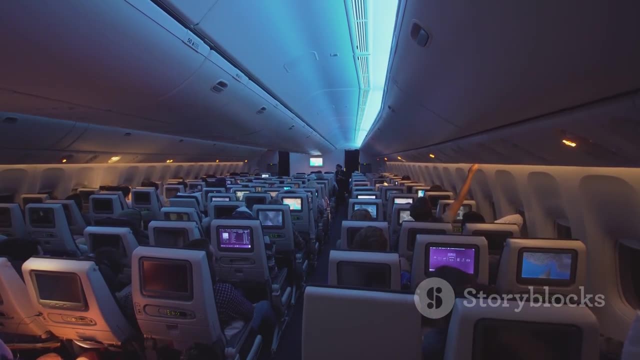 or the strongest, but it gets the job done And it does it well. For decades it has carried the weight of passengers and cargo across the globe, proving its worth time and time again. But what makes aluminum so suitable for aircraft? Well, let's delve a little deeper. 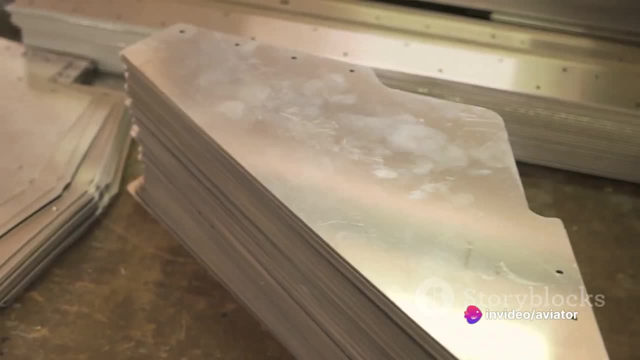 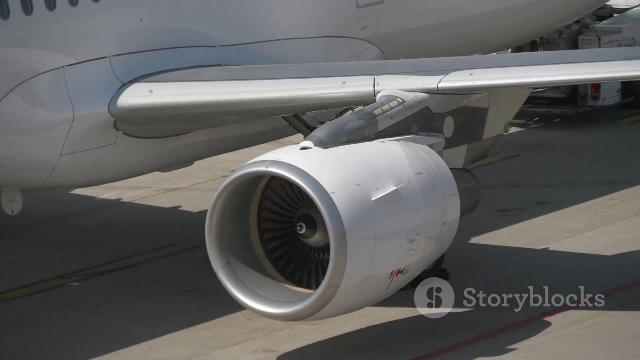 Aluminum is a metal that's known for its lightweight. In aviation, every ounce matters. The lighter the aircraft, the less fuel it needs, which means lower costs and less environmental impact. So a lightweight material like aluminum is a big win for aircraft manufacturers. But 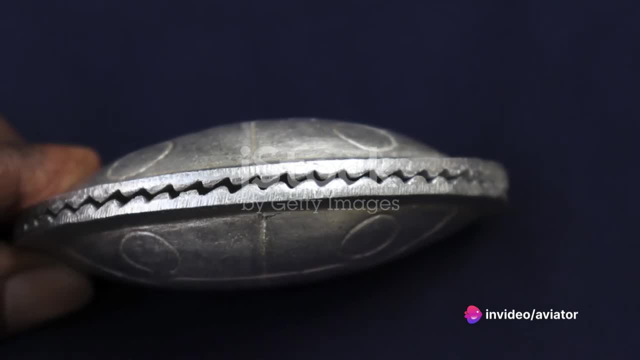 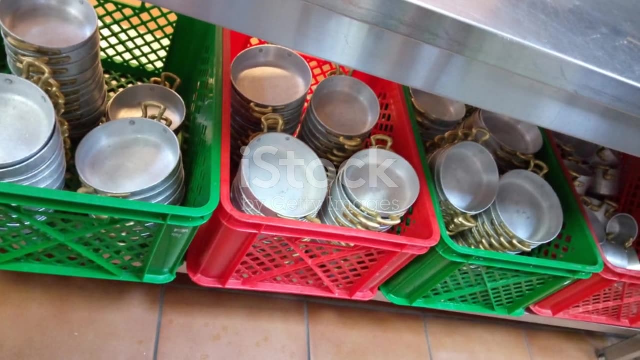 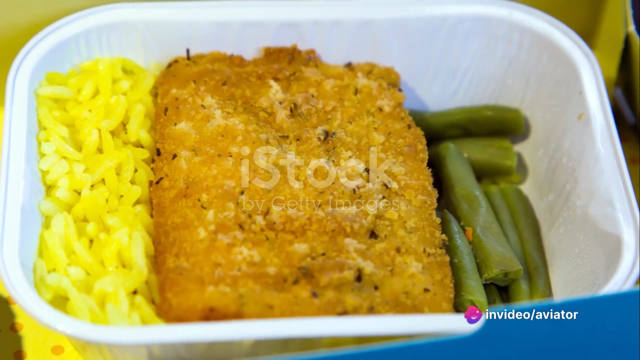 that's not all. Aluminum is also relatively easy to work with. It can be shaped into complex forms, making it ideal for creating the sleek aerodynamic shapes we associate with modern aircraft. From the fuselage to the wings, aluminum has been instrumental in the design and construction. 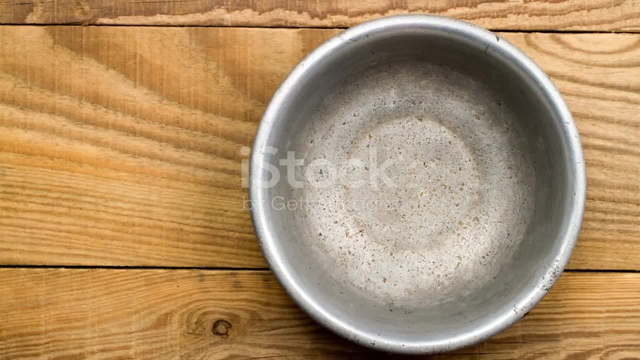 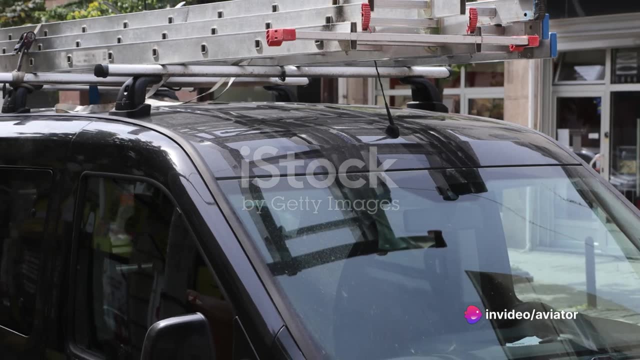 of many aircraft components, And let's not forget about the engine. Aluminum's heat resistance makes it a good choice for engine components where temperatures can get extremely high. Its strength and durability can handle the intense pressures and stresses that come with powering an aircraft through. 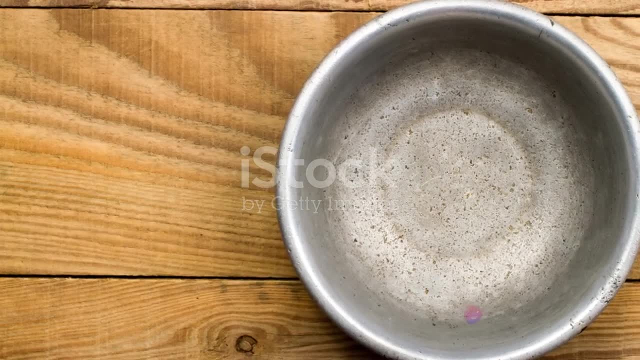 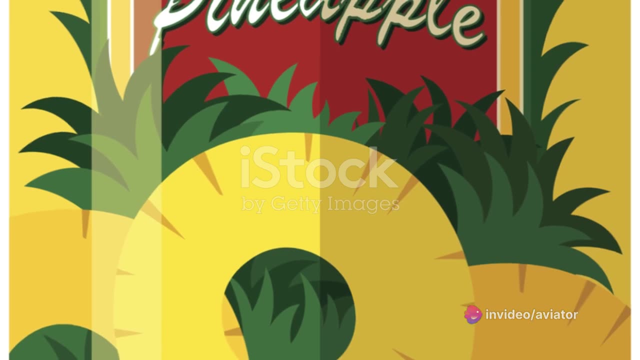 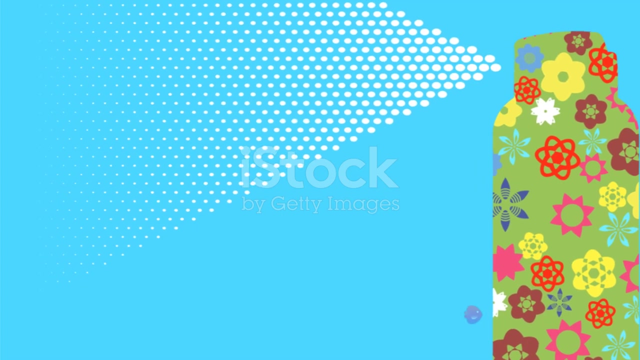 the skies. In short, aluminum has been a trusted ally in the aviation industry, playing a crucial role in the design and construction of aircraft. It's a material that stood the test of time, proving its worth in countless flights around the globe. So aluminum, with its marvelous properties, has been the workhorse in the aviation industry. 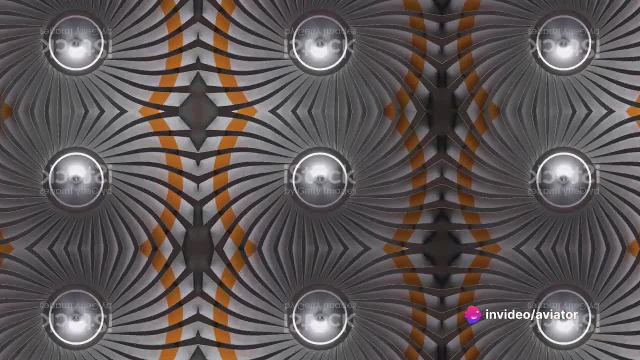 It has carried us through the skies and it continues to do so today. Enter titanium. Aluminum is a metal that's known for its light weight. Aluminum's heat resistance makes it a good choice for aircraft manufacturers. Aluminum's heat resistance makes it a good choice for. 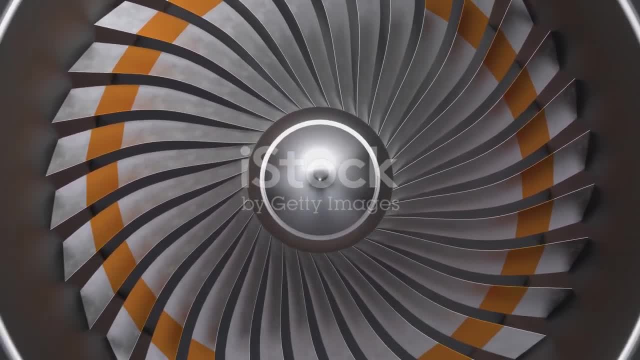 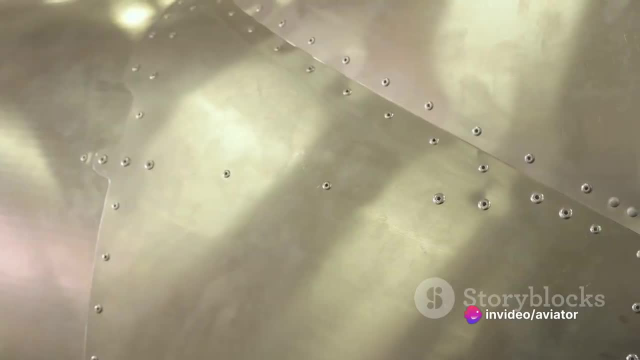 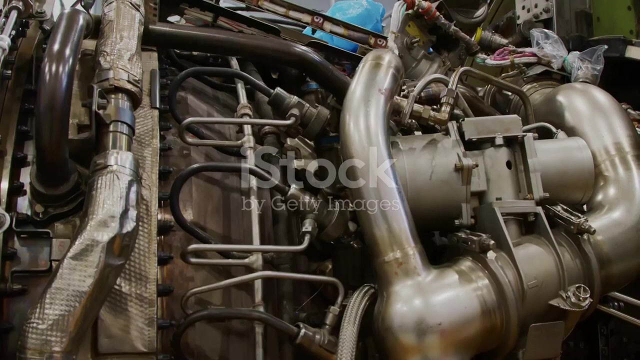 aircraft manufacturers. Aluminum's heat resistance makes it a good choice for aircraft manufacturers. The magic metal with an exceptional strength-to-weight ratio, Titanium, through its unique properties, has revolutionized the way we think about aircraft materials. This is no ordinary metal — it's a champion in the realm of strength and weight, A balance so crucial in the world. 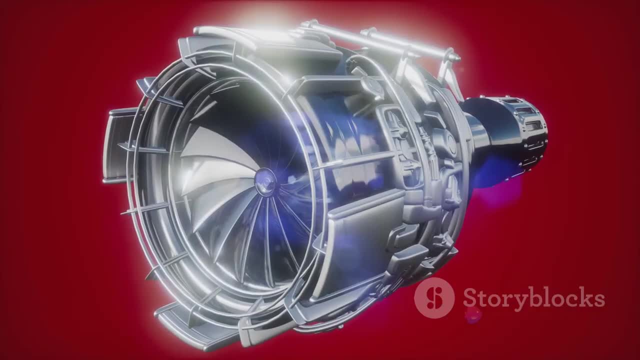 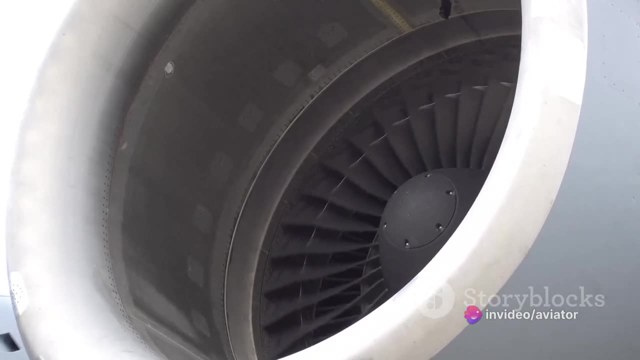 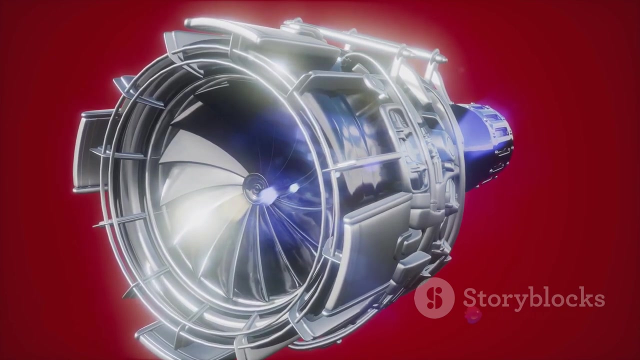 of aviation, Let's delve into the heart of an aircraft: the engine. This is where titanium truly shines. Engine parts face extremely high temperatures and pressures, And this is where the strength comes into play. It withstands the rigors of the engine environment effortlessly without. 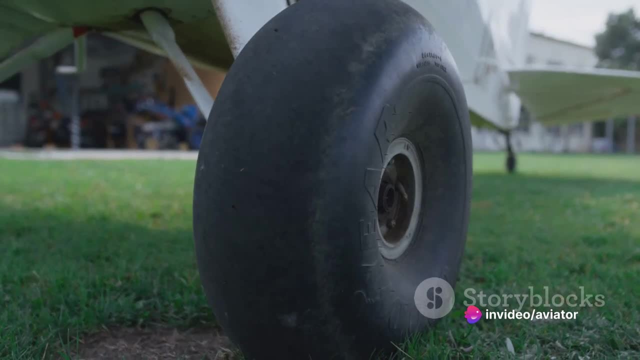 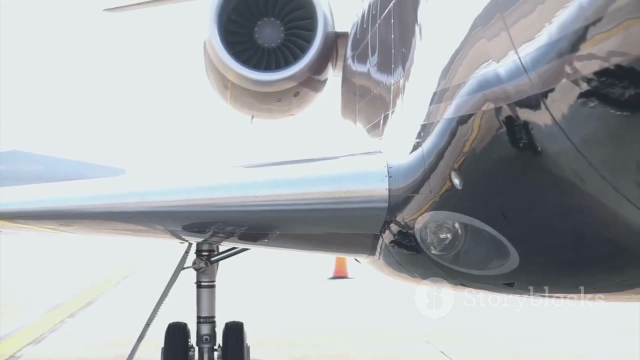 adding excessive weight. Now think about the landing gear. Imagine the impact when an aircraft touches down. It's like a ballet dancer landing after a tremendous leap. The landing gear absorbs this shock. and here again, titanium proves its worth: Its high. 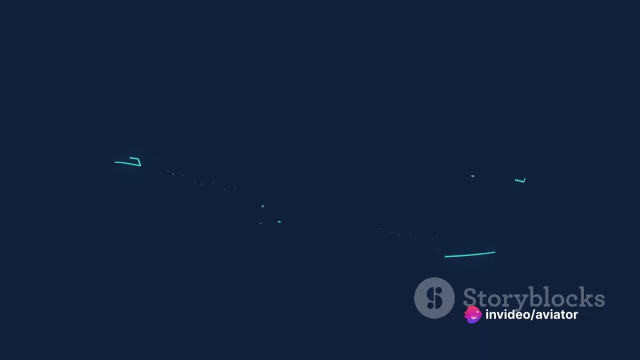 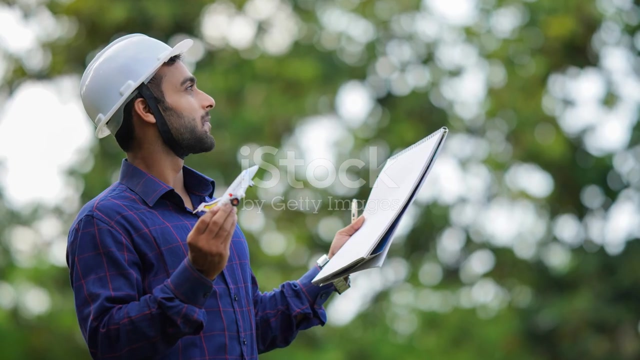 strength and lightness make it the ideal choice for this high-stress application. But the applications of titanium don't stop there. It's also used in critical structural elements in the aircraft. These are the parts that bear the brunt of the forces during flight. and they need to be as strong as possible, yet as light as a feather. Titanium fits this bill perfectly, providing the required strength without the weight penalty. But every superhero has its kryptonite, and for titanium it's cost. Titanium is expensive to mine, refine. 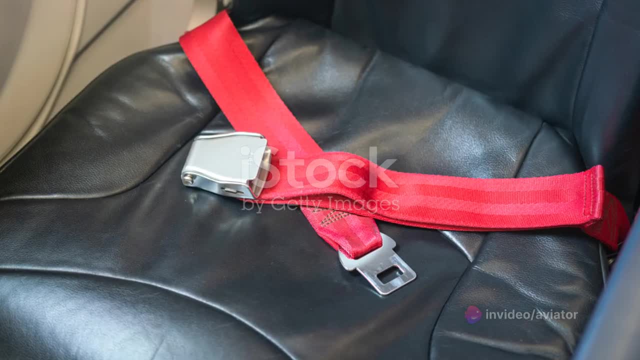 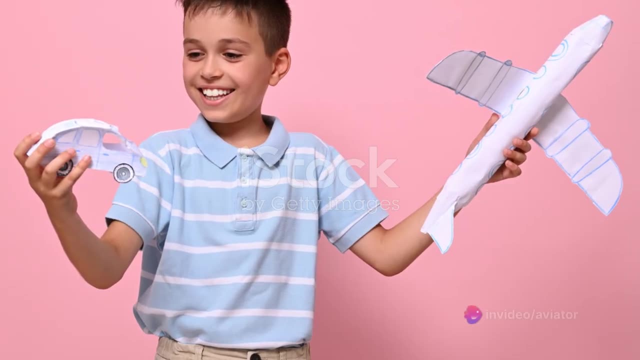 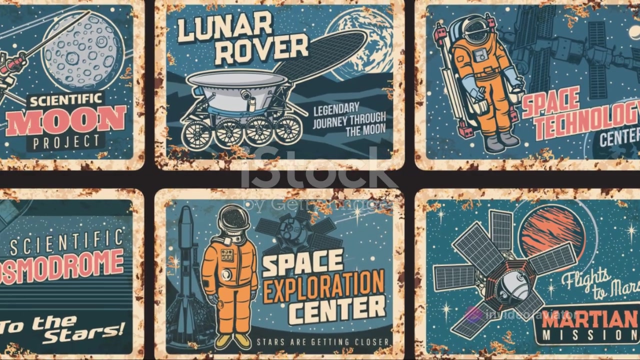 and process. This makes it a costly option compared to other materials. But here's the thing: In aviation, safety and performance are paramount, And if you use titanium in critical areas enhances these aspects, then the cost is justified. Despite being costly, titanium's unparalleled strength and lightness make it a key player in high-performance. 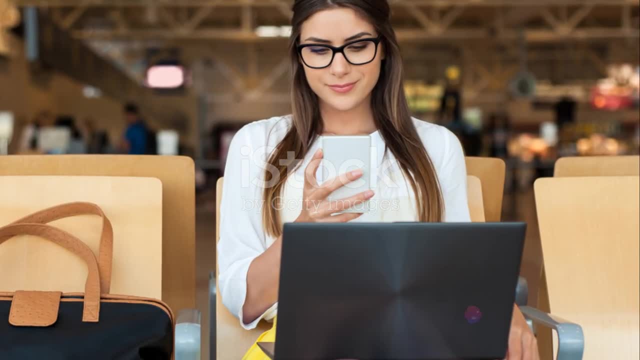 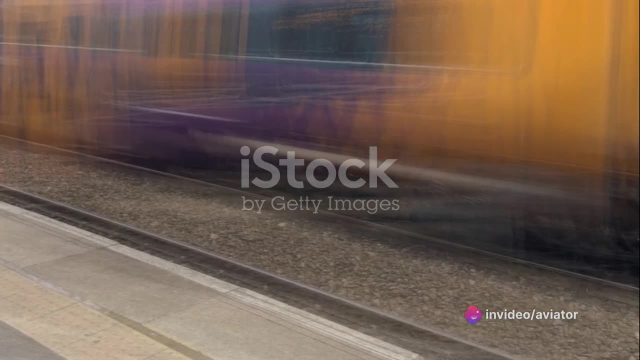 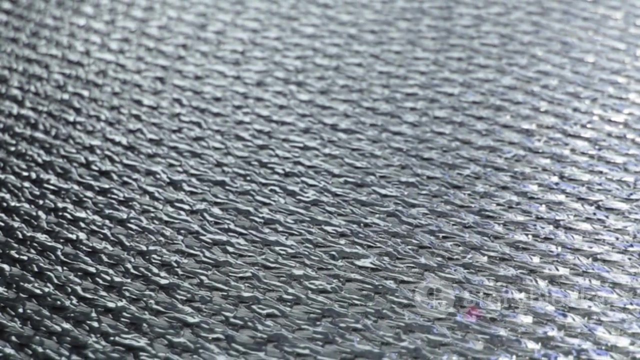 aircraft. So next time you marvel at a jet streaking across the sky, remember that within its sleek form, titanium is doing its magic, helping it soar high and fast, embodying the perfect marriage of strength and weight. Now let's dive into the world of composites, where carbon and glass fibers are reinventing. 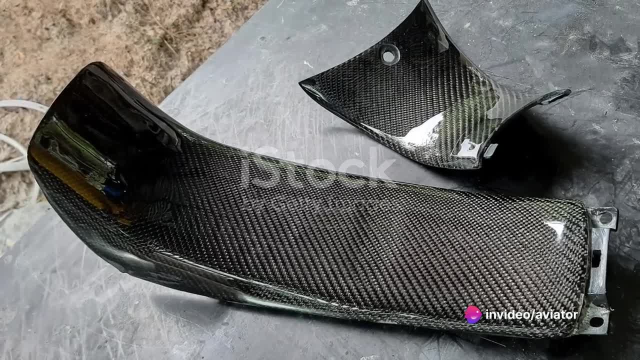 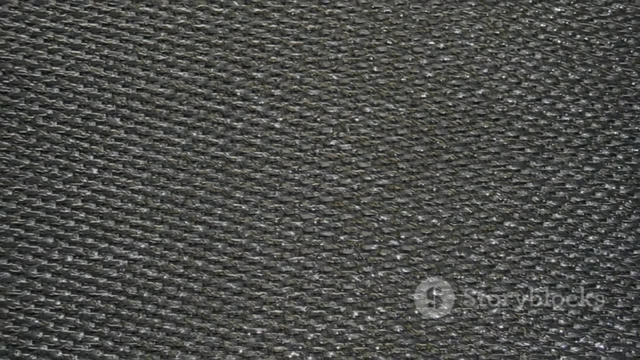 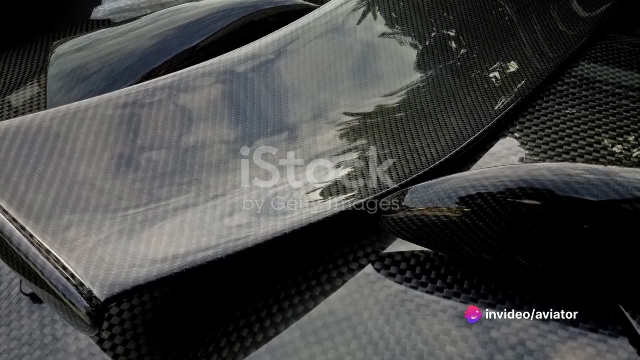 flight Composites, as the name suggests, are materials made by combining two or more distinct elements to create a superior product. In the world of aviation, carbon fiber and glass fiber composites have become game-changers, revolutionizing the way we design and build aircraft. 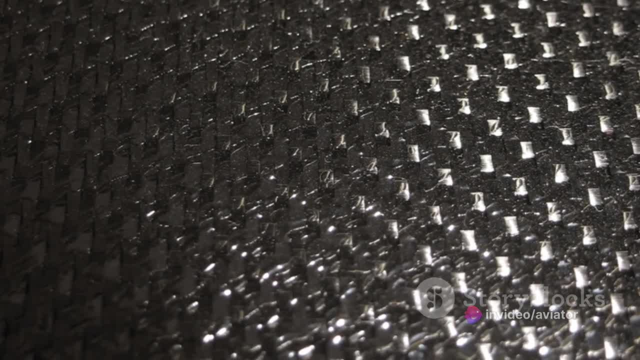 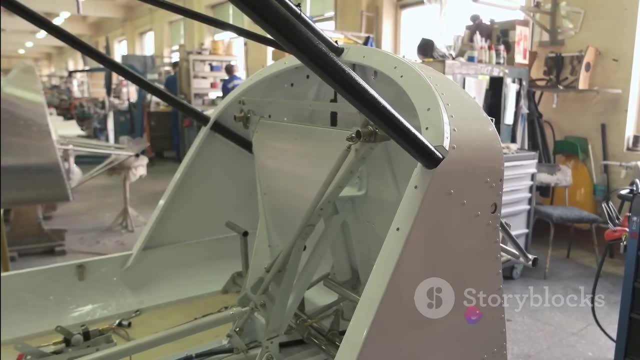 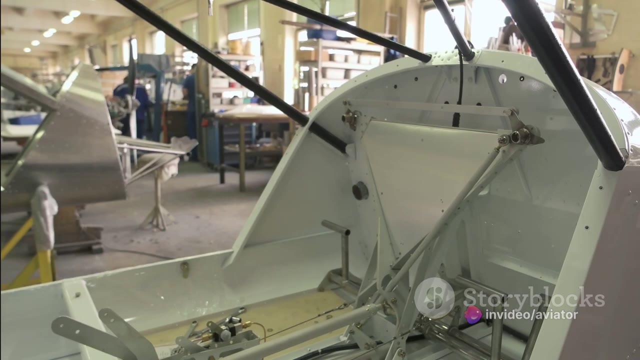 First up, carbon fiber composites. These are made up of carbon fibers, which are incredibly thin strands of carbon atoms embedded in a matrix of epoxy resin. The result: A material that is both lightweight and high-strength. This makes carbon fiber composites ideal for critical structural components of an aircraft. 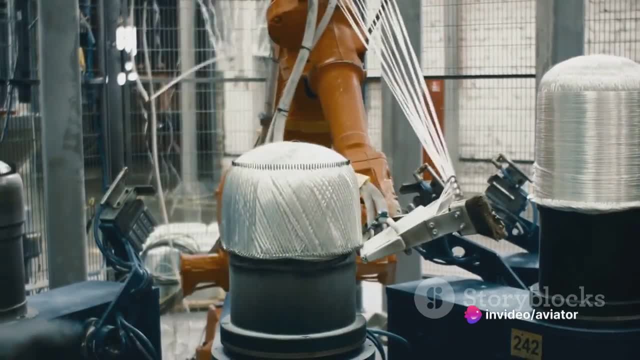 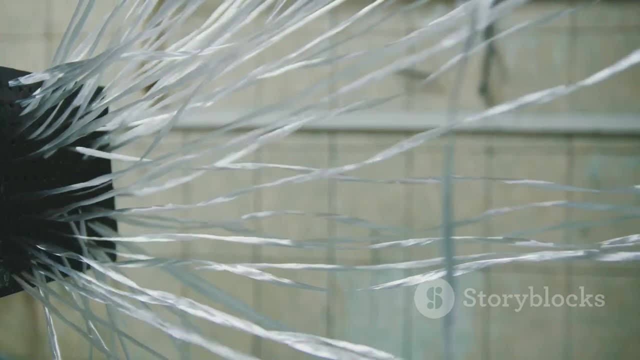 such as the wings and tail sections. And, as an added bonus, these composites are highly corrosion-resistant, a trait that gives them a significant edge in the demanding environment of aviation. But the story of composites doesn't end with carbon fiber, Glass fiber composites made 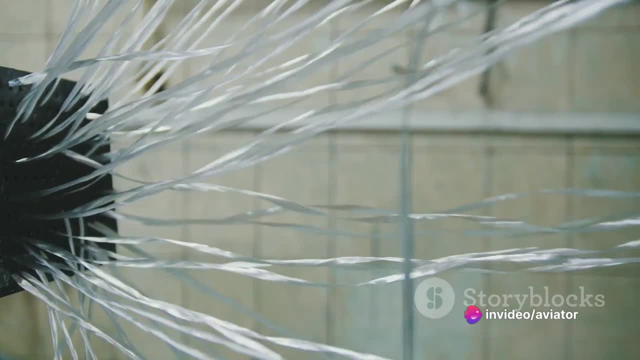 up of glass fibers woven into a polymer matrix are another vital component of carbon fiber. Carbon fiber composites made up of glass fibers woven into a polymer matrix are another vital component of carbon fiber. While they might not be as stiff as their carbon fiber counterparts, they have a crucial 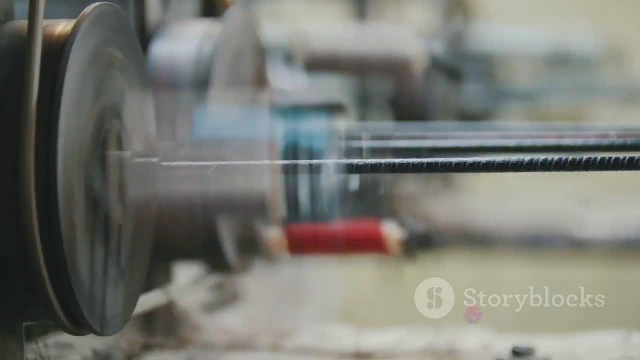 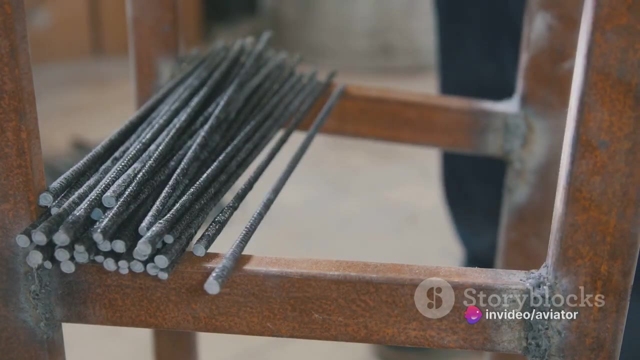 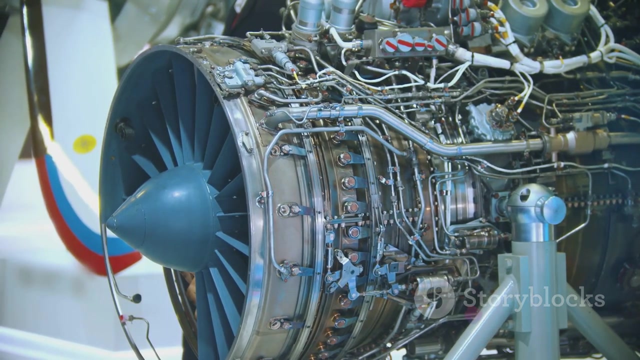 advantage: They are more impact-resistant. This quality makes them particularly useful for parts of the aircraft that are less critical structurally but need to withstand potential impacts, like interior panels and fairings. In both cases, these composites offer significant weight savings compared to traditional metals. 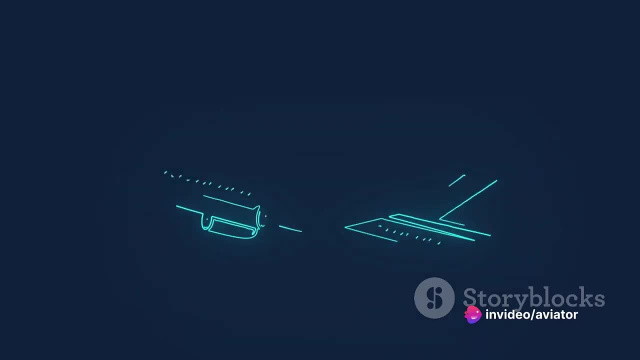 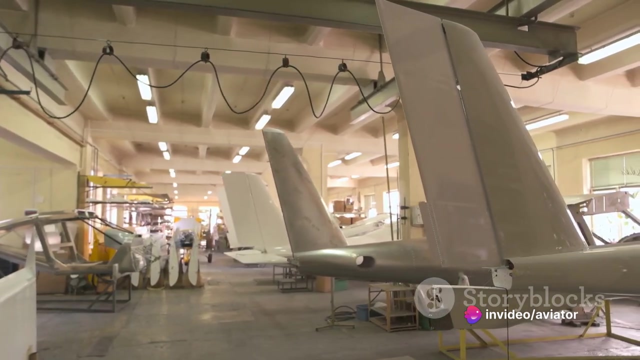 This lighter weight translates directly into fuel efficiency, making flights more cost-effective to the environment. Plus, the versatility of composites lets engineers mold them into complex shapes, opening up new possibilities in aerodynamic design. But why stop at carbon and glass fibers? Engineers are continually pushing the boundaries, exploring. 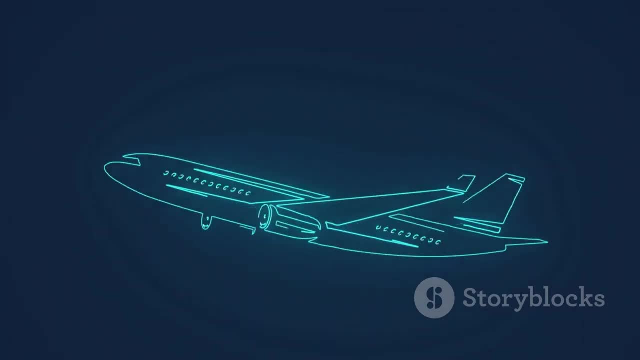 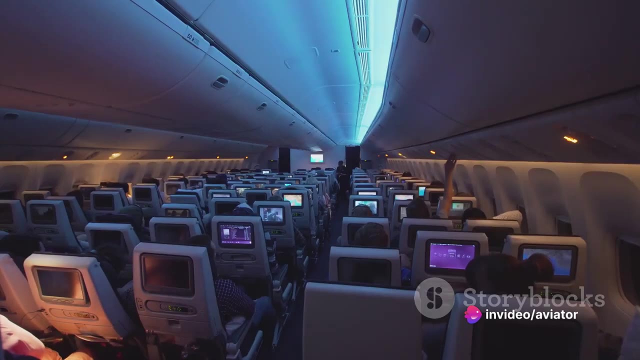 other fiber materials and tweaking the resin matrix to create composites with even better properties. The quest for the perfect material never ends and the potential for innovation is boundless. So next time you see a sleek, modern jet airliner, don't forget to subscribe to our YouTube channel. 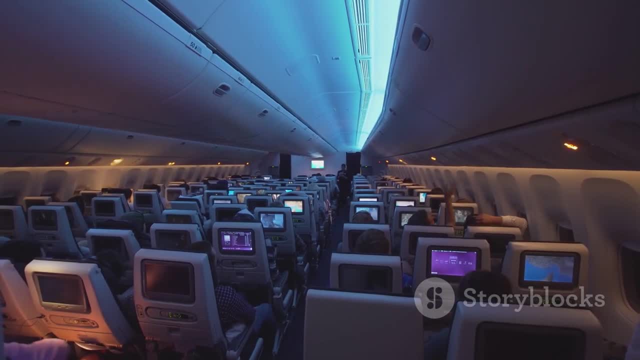 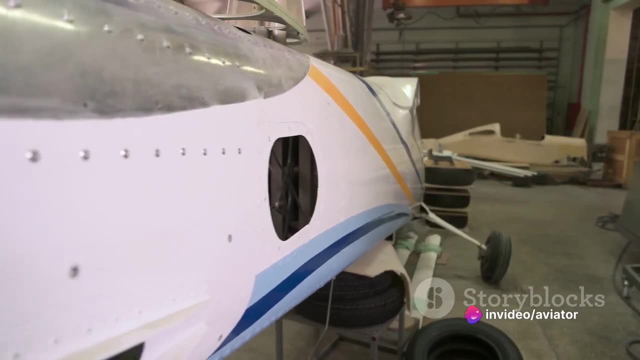 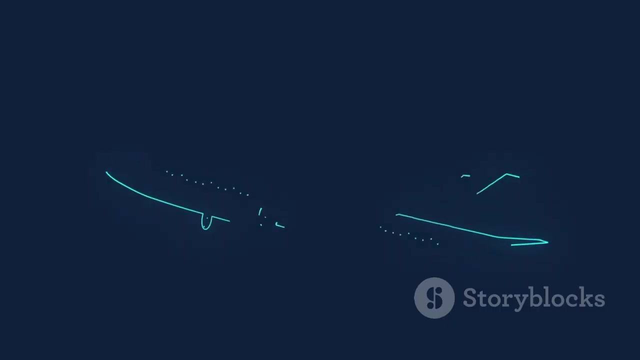 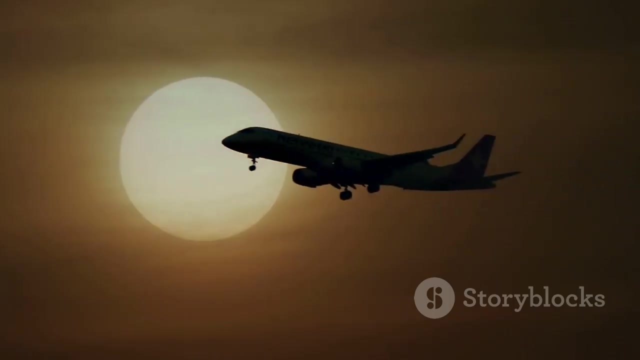 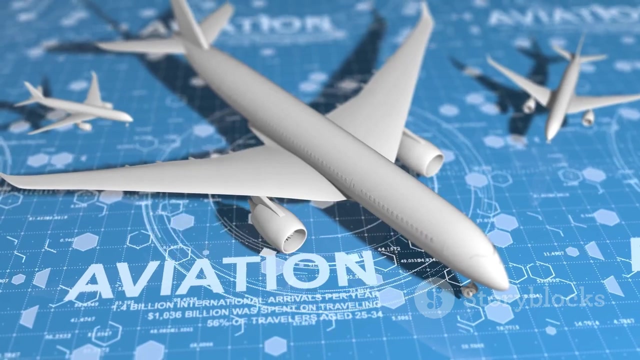 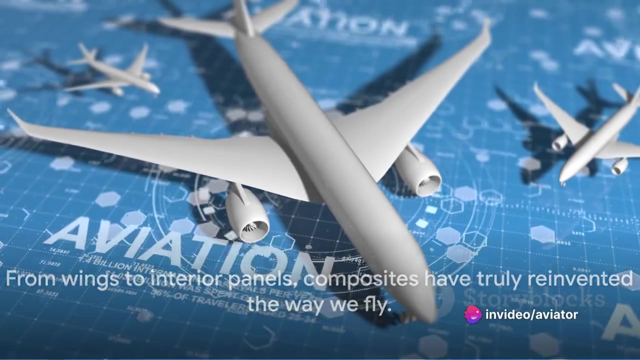 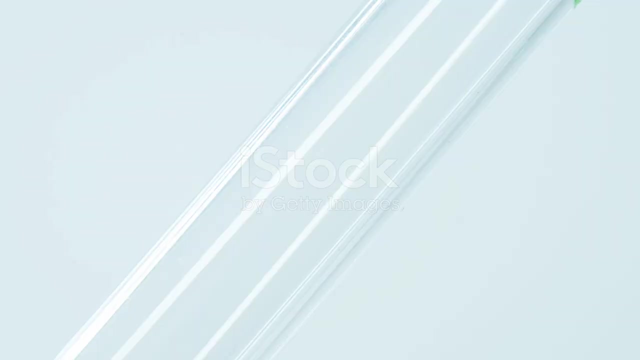 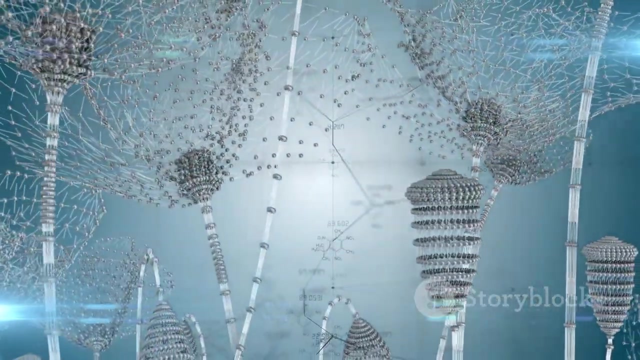 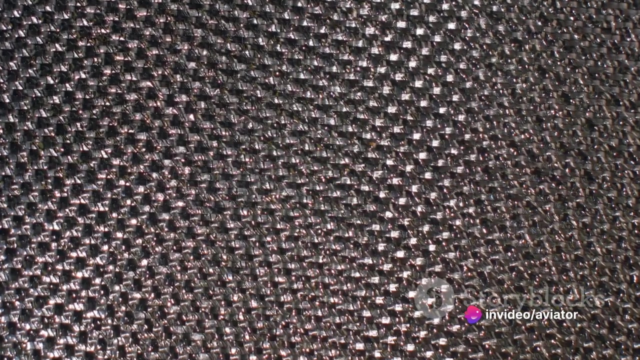 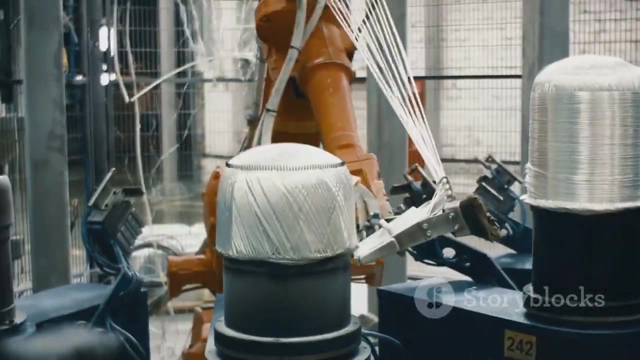 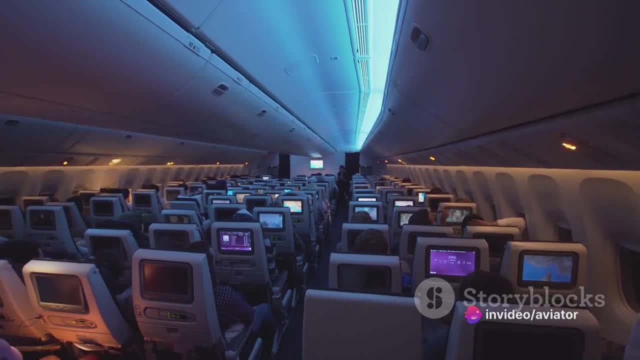 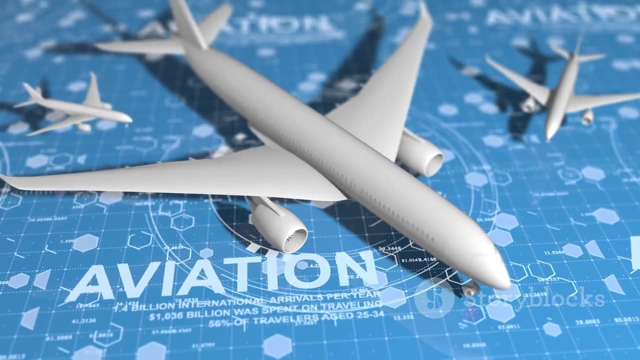 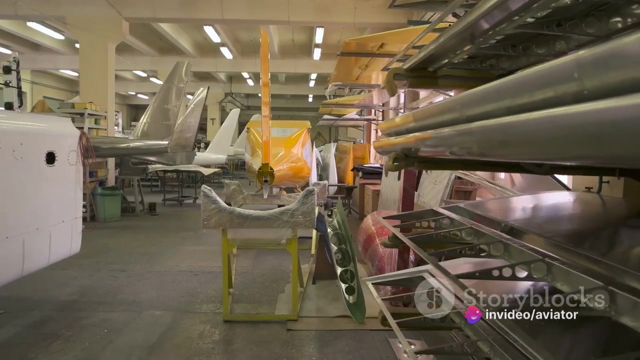 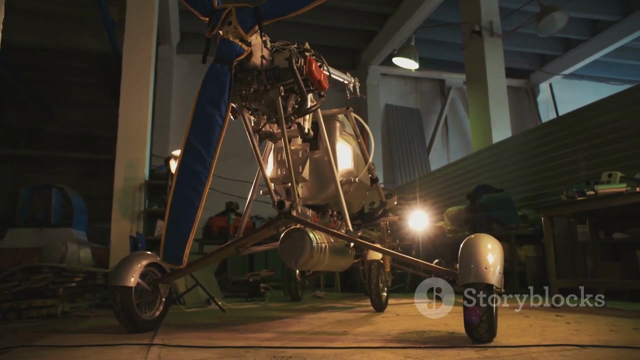 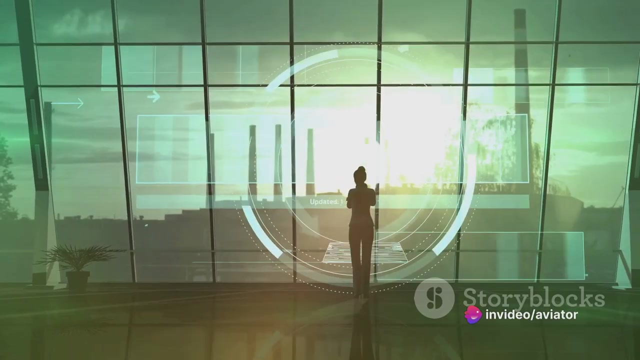 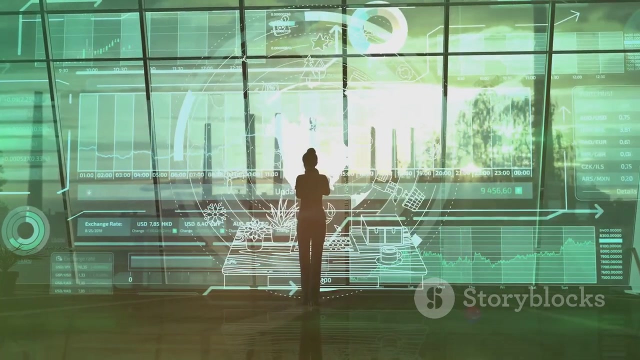 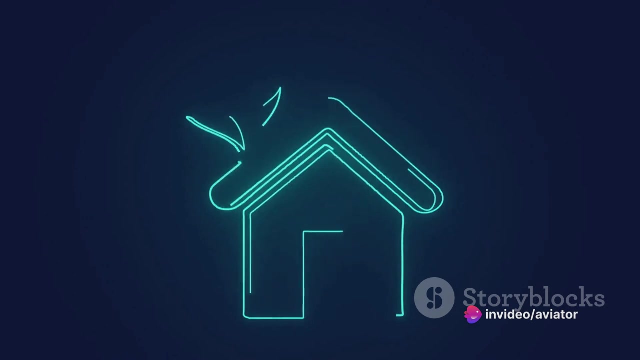 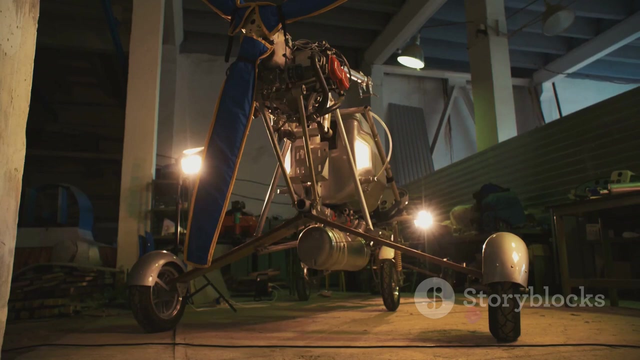 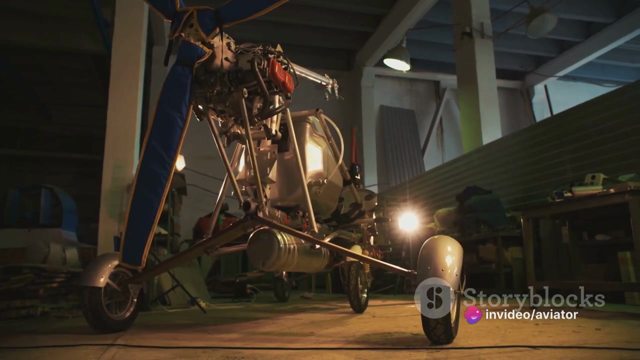 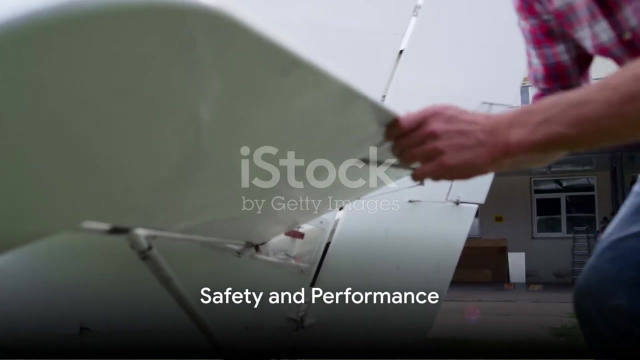 Thanks for watching and we'll see you in the next video. Thanks for watching and we'll see you in the next video. and recyclability are paving the way for a greener aviation industry. Choosing the right material for an aircraft is a balancing act. 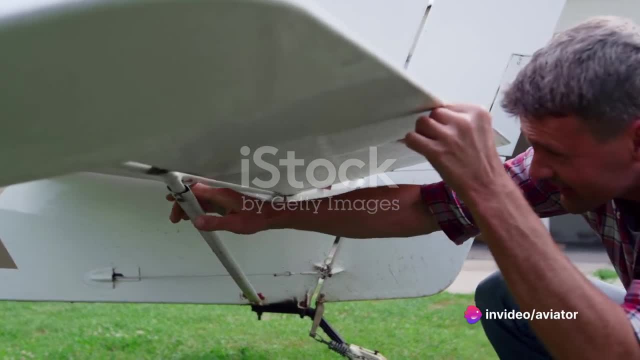 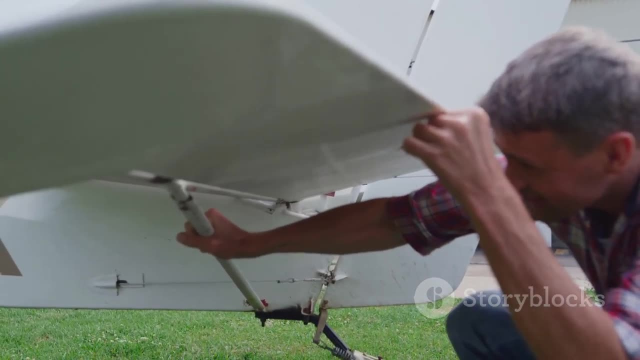 Engineers must weigh a multitude of factors, from the material's weight and strength to its cost and availability. But beyond these considerations, there are two crucial aspects they cannot overlook: safety and performance. When we talk about safety, we're referring to a material's durability.